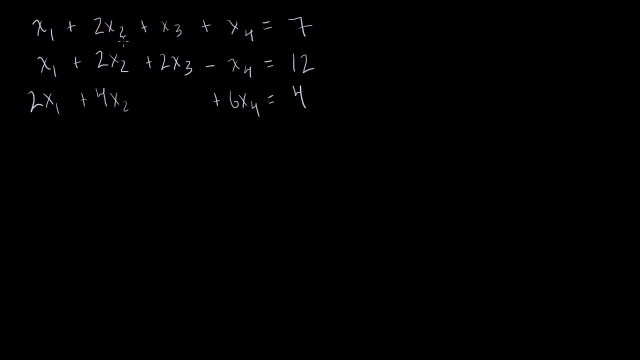 matrices, and the matrices are really just arrays of numbers that are shorthand for this system of equations. So let me create a matrix here, So I could just create a coefficient matrix, where the coefficient matrix would just be. Let me write it neatly: 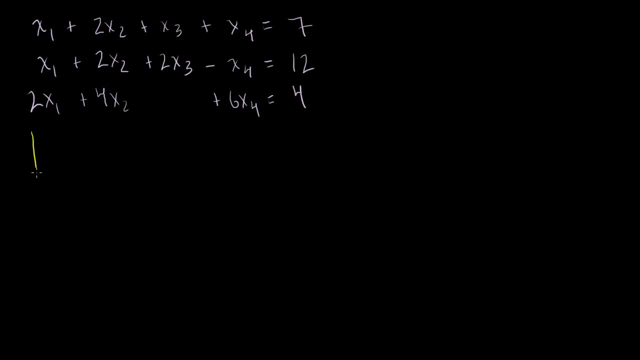 The coefficient matrix would just be The coefficients on the left-hand side of these linear equations. So the coefficient there is 1.. Coefficient there is 1.. Coefficient there is 2.. And you have 2,, 2,, 4.. 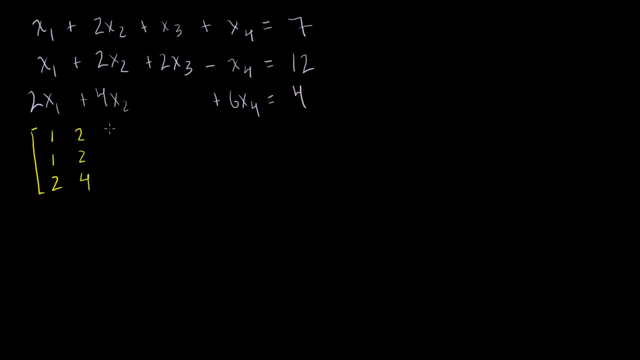 2, 2, 4.. 1, 2, 0.. There's no coefficient on the x3 term here because there's no x3 term there. So we'll say the coefficient on the x3 term there is 0. 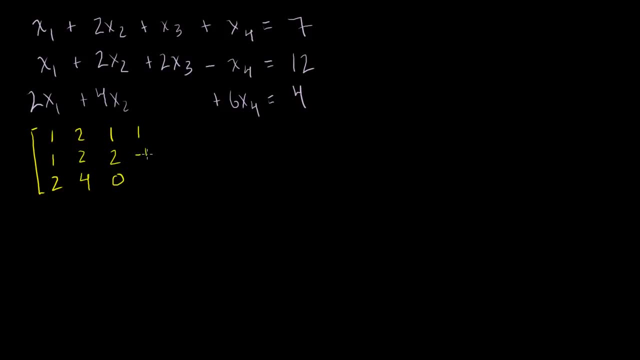 And then we have 1 minus 1.. 1 minus 1. Minus 1 and 6.. Now if I just did this right there, that would be the coefficient matrix for this system of equations right there. but what I want to do is I want to augment it. 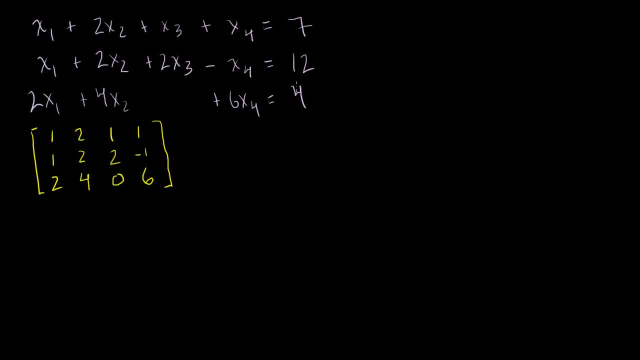 I want to augment it with what these equations need to be equal to. So let me augment it, And what I'm going to do is I'm going to draw a little line here and write the 7,, the 12, and the 4.. 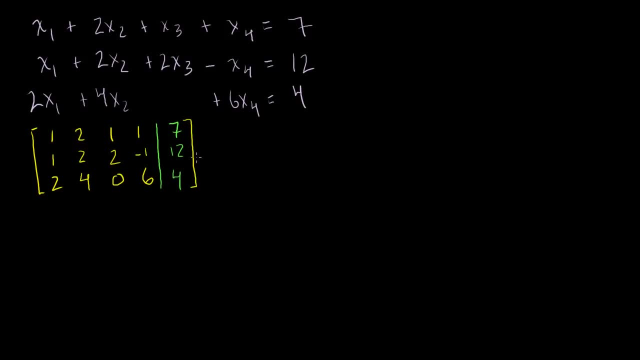 And I think you can see that whatever this right here is, it's just another way of writing this And just by the position, we know that these are the coefficients on the x1 terms. We know that these are the coefficients on the x2 terms. 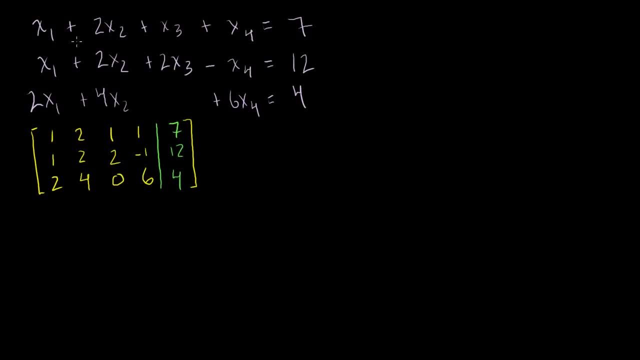 And what this does. it really just saves us from having to write x1 and x2 every time, But we can essentially do the same operations on this that we otherwise would have done on that. So what we can do is we can replace any equation with that. 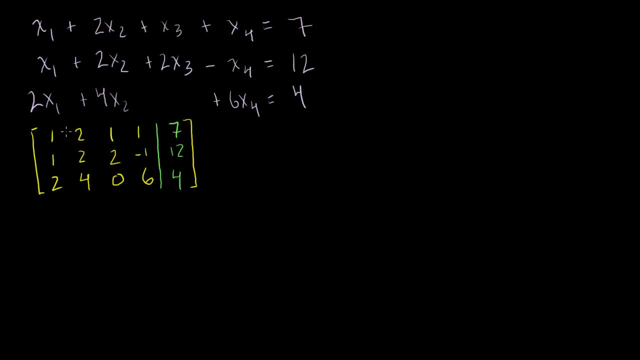 equation times, some scalar multiple plus another equation. We can divide an equation or multiply an equation by a scalar. We can subtract them from each other, We can swap them. So let's do that in an attempt to solve this equation. So the first thing I want to do, just like I've done in the 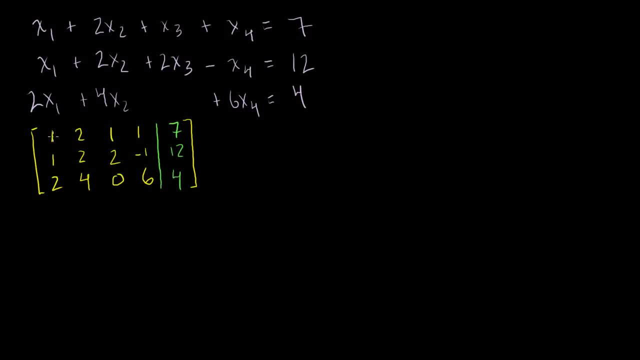 past is. I want to get this equation to the form of where, if I can, I have a 1,, my kind of leading coefficient in any of my rows is a 1, and that every other entry in that column is a 0.. 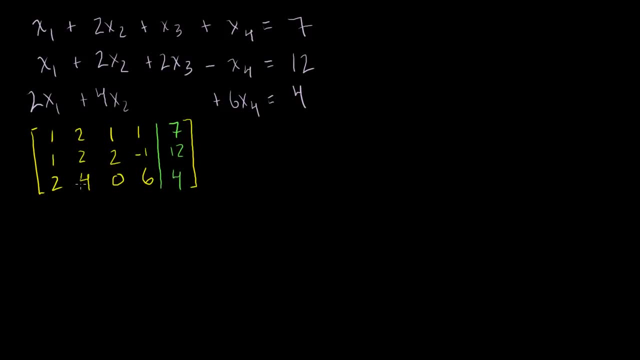 And in the past I made sure that every other entry below it is a 0. That's what I was doing in some of the previous videos when we tried to figure out if things were linearly independent or not. But now I'm going to make sure that if there's a 1,, if there's 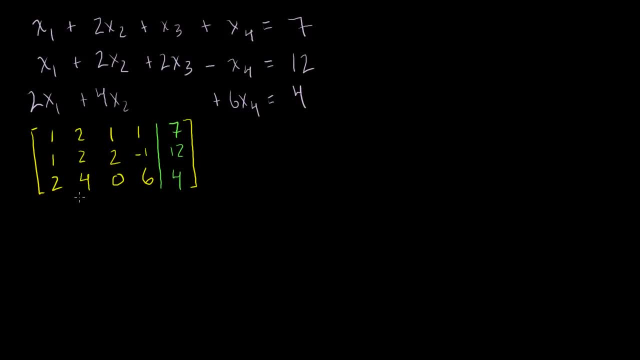 a leading 1 in any of my rows that everything else in that column is a 0. And that form I'm doing is called reduced row- echelon form. Let me write that Reduced row- echelon form And if we call this augmented matrix, 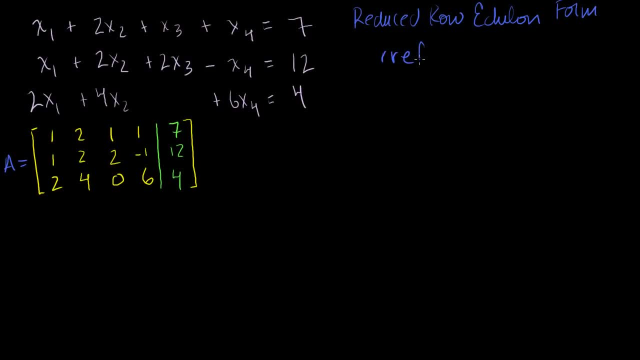 matrix A, then I want to get it into the reduced row echelon form of matrix A And matrices. the convention is just like vectors: you make them nice and bold, but use capital letters instead of lowercase letters, And we'll talk more about how matrices relate to vectors in. 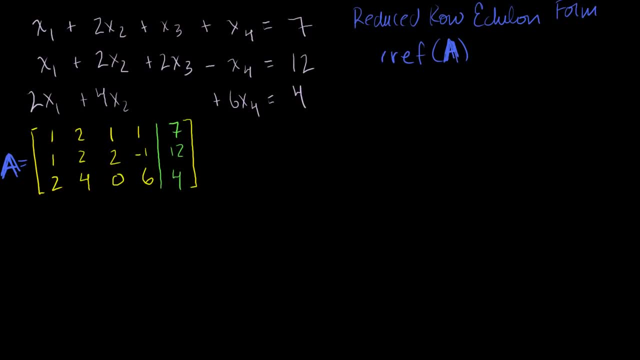 the future. But let's just solve this system of equations. So the first thing I want to do is, in an ideal world, I would get all of these guys right here to be 0. So let me replace this guy With that guy, with the first entry minus the second entry. 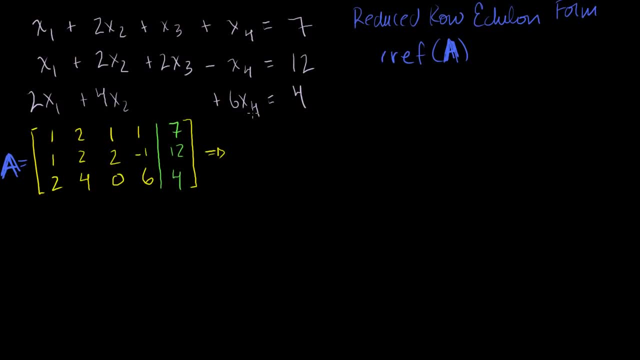 So let me do that. So I am just going to. the first row isn't going to change, it's going to be 1, 2,, 1, 1, and then I get a 7 right there. that's my first row. 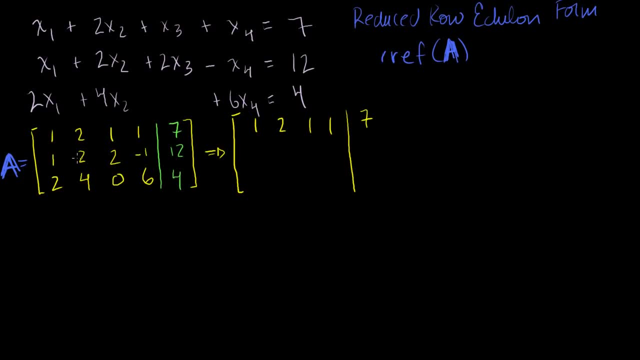 Now the second row. I'm going to replace it with the first row minus the second row. So what do I get? 1 minus 1 is 0.. 2 minus 2 is 0.. 1 minus 2 is minus 1.. 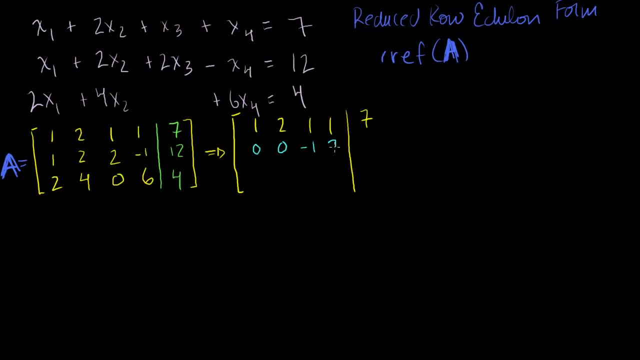 And then 1 minus minus 1 is 2.. That's 1 plus 1.. And then 7 minus 12 is minus 5.. All right, now I want to get rid of this row here. I don't want to get rid of it. I want to get rid of this 2. 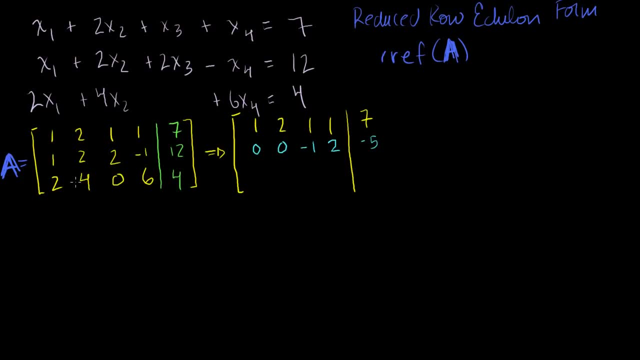 right here. I want to turn it into a 0.. So let's replace this row with this row minus 2 times that row. So what I'm going to do is this row minus 2 times the first row and I'm going to replace this row with that. 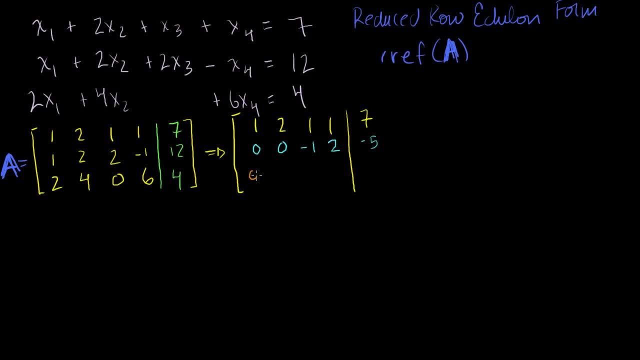 So 2 minus 2 times 1 is 0.. That was the whole point. 4 minus 2 times 2 is 0.. 0 minus 2 times 1 is minus 2.. 6 minus 2 times 1 is 6 minus 2, which is 4.. 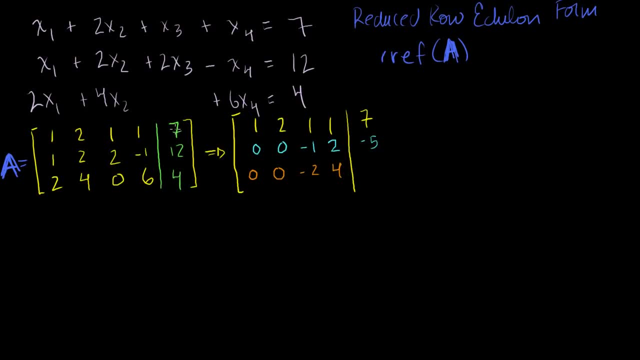 And then 4 minus 2 times 7.. OK, 7 is 4 minus 14,, which is minus 10.. All right now, what can I do next? Well, ideally I don't have any. well, this guy, you can. 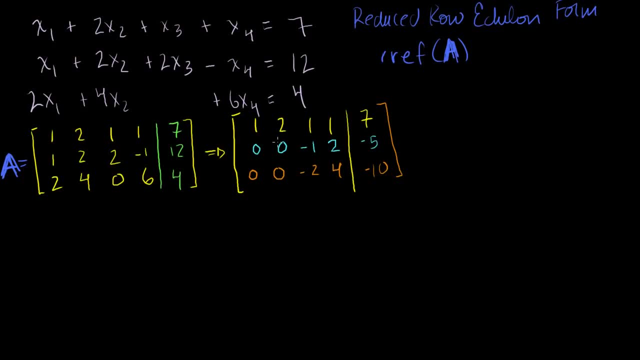 kind of see. this row is kind of well. we'll talk more about what this row means. when all of a sudden, it's just all been zeroed out. There's nothing here. If I had a non-zero term here, then I'd want to zero this guy. 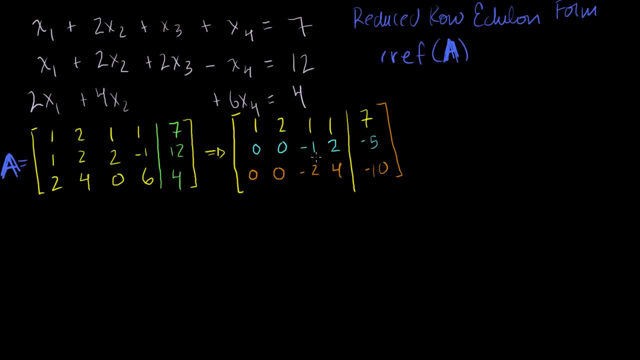 out, although it's already zeroed out. So I'm just going to move over to this row. So the first thing I want to do is I want to make sure that I'm going to make this leading coefficient here a 1.. So what I want to do is I'm going to multiply this entire 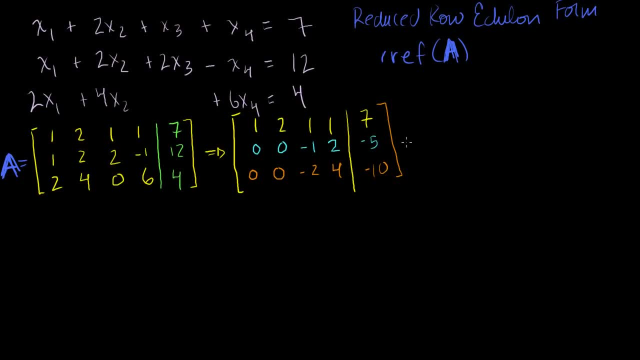 row by minus 1.. So if I multiply this entire row times minus 1,- in fact I don't even have to rewrite the matrix- This becomes plus 1, minus 2, plus 5.. I think you can accept that. 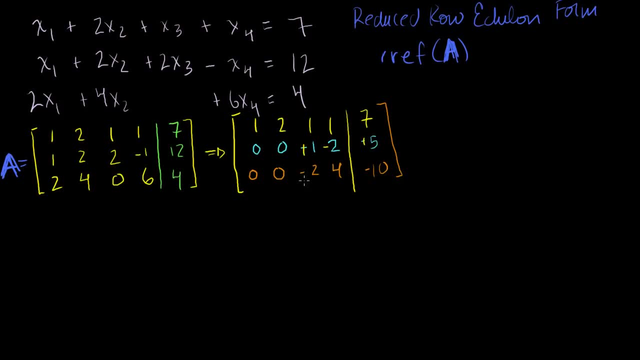 All right now what can we do? Well, let's turn this right here into a 0.. So let me rewrite. Let me write my augmented matrix in the new form that I have. So I'm going to keep the middle row the same this time. 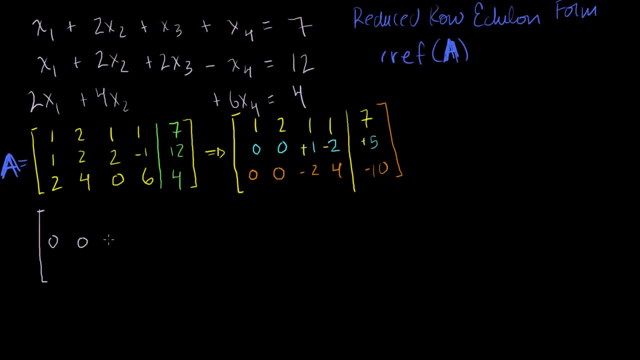 So my middle row is 0, 0,, 1, minus 2, and then it's augmented and I get a 5 there, And what I want to do is I want to eliminate this minus 2 here. So why don't I add this row to 2 times that row, right? 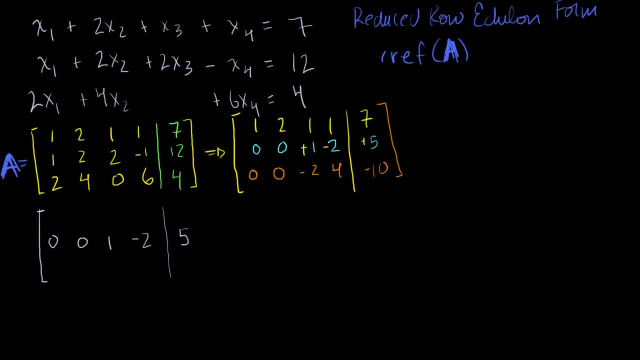 Then I would have minus 2 plus 2, and that'll work out. So what do I get? I get a. well, these are just leading 0's, and then I have minus 2 plus 2 times 1.. 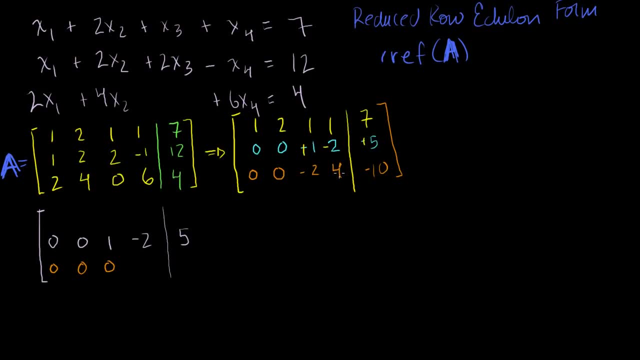 Well, that's just 0.. 4 plus 2 times minus 2.. 4 plus 2 times minus 2.. That's minus 4.. So that's 4 plus minus 4.. That's 0 as well. 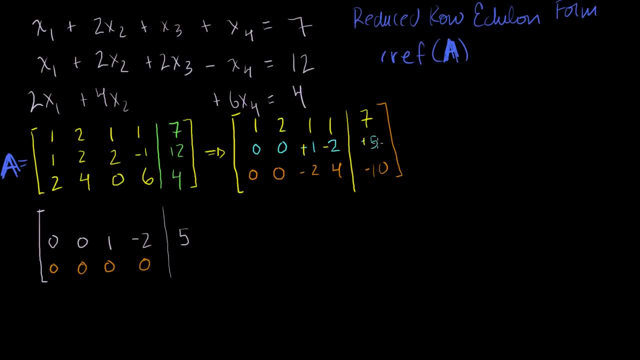 And then you have minus 10 plus 2 times 5. Well, that's just minus 10.. Plus 10,, which is 0. So that one just got zeroed out And what I want to do, and normally when I just did. 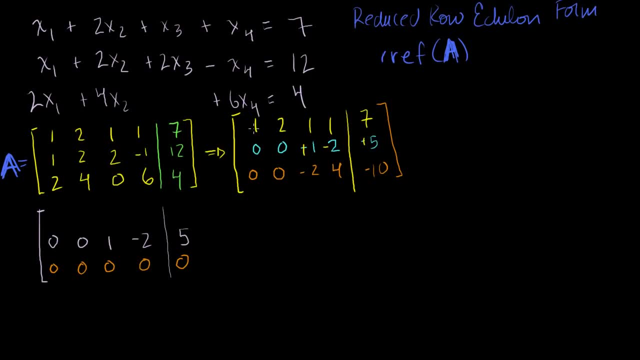 regular elimination. I was happy just having the situation where I just had these leading 1's. everything below it were 0's, but I wasn't too concerned about what was above our 1's. But what I want to do is I want to make those into a 0 as well. 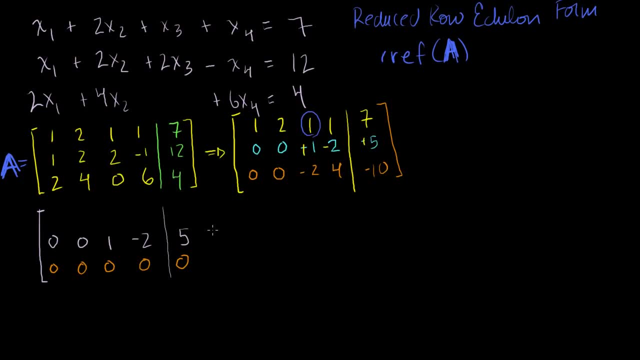 So I want to make this guy a 0 as well. So what I can do is I can replace this first row with that first row minus the second row. So what is 1 minus 0?? Well, that's just 1.. 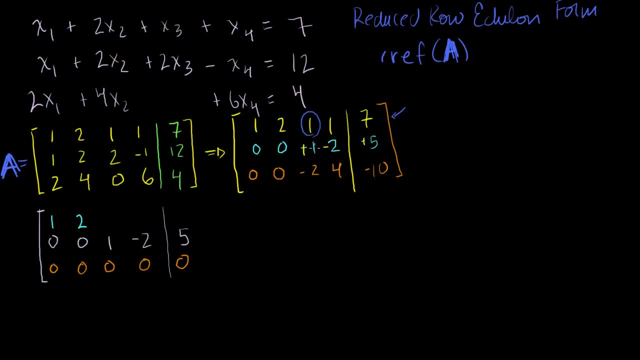 2 minus 0 is 2.. 1 minus 1 is 0.. 1 minus minus 2 is 3.. 7 minus 5 is 2.. And there you have it. We have our matrix in reduced row echelon form. 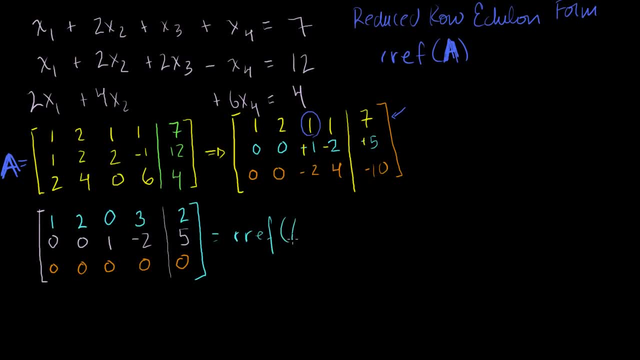 This is the reduced row echelon form of our matrix. I'll write it in bold- Of our matrix A, right there. And you know it's in reduced row, echelon form because all of your leading 1's in each row. So what are my leading 1's in each row? 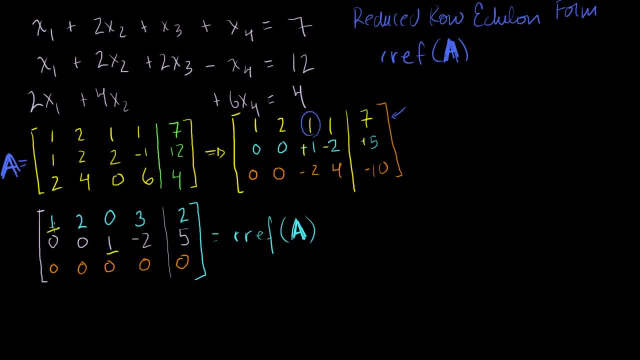 I have this one and I have that one. They're the only non-zero entry in their columns and these are called the pivot entries. Let me label that for you. That's called a pivot entry- Pivot entry. They're the only non-zero entry in their respective columns. 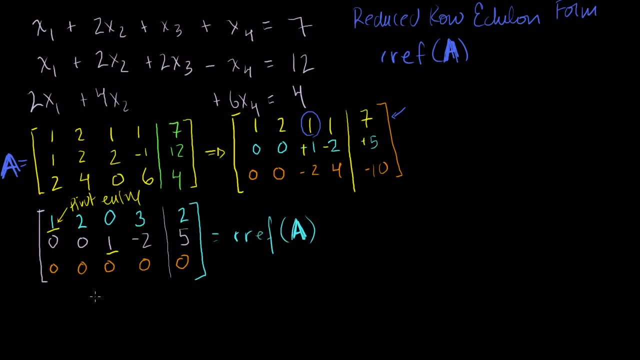 If I have any zeroed out rows- and I do have a zeroed out row, it's right there. So this is a zeroed out row. Just the style or just the convention? is that for reduced row, echelon form, that has to be your last row? 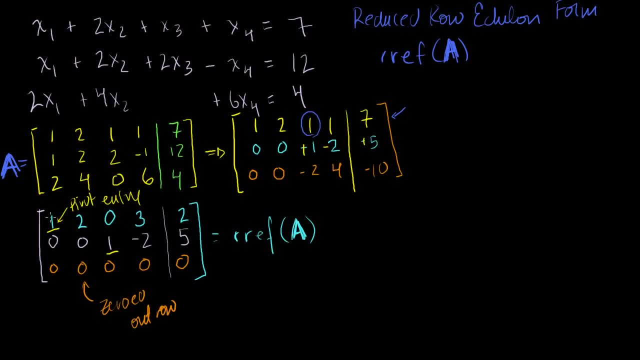 So we have. the leading entries are the only. they're all 1.. That's one case. You can't have this a 5.. You'd want to divide both. You would want to divide that equal. You'd want to divide the equation by 5 if this was a 5.. 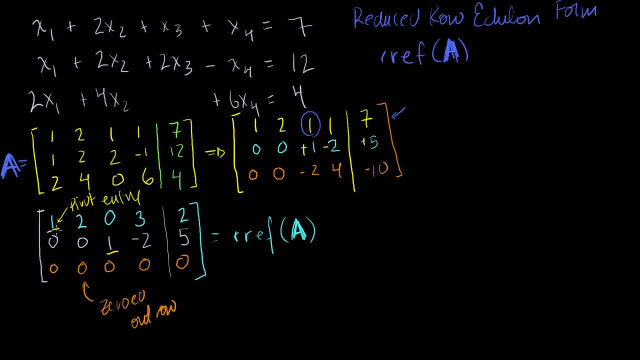 So your leading entries in each row are: 1. That the leading entry in each successive row is to the right of the leading entry of the row before it. This guy right here is to the right of that guy. This is just the style, the convention of reduced row. 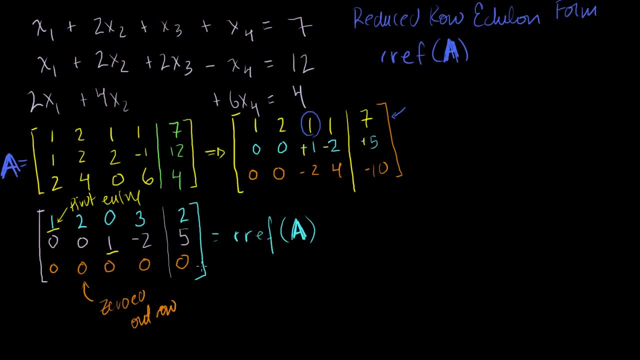 echelon form, And if you have any zeroed out rows, it's in the last row. And then finally, of course- and I think I've said this multiple times- this is the only non-zero entry in the row. Now, what does this do for me? 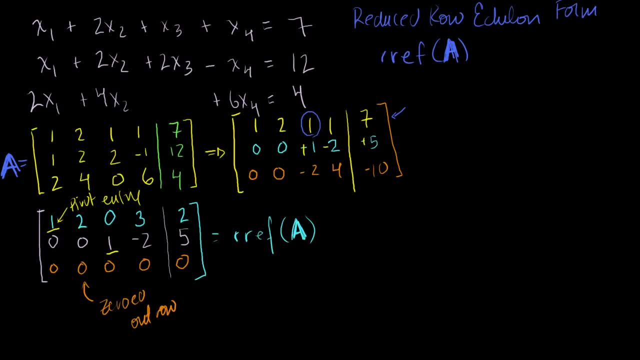 Well, now I can go back from this world, back to my linear equations, Because we remember that these were the coefficients on x1.. These were the coefficients on x2.. These were the coefficients on x3, on x4.. And then these were my constants out here. 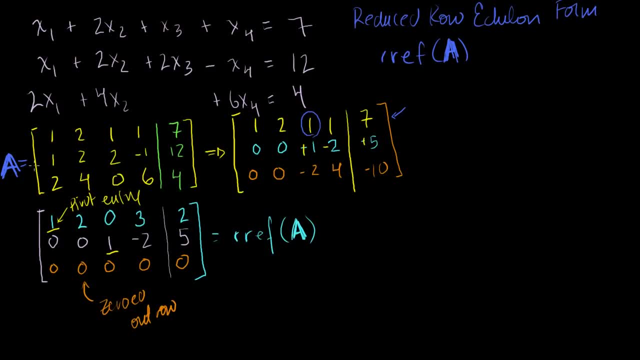 So I can rewrite this system of equations using my reduced row echelon form as x1 plus 2x2.. There's no x3 there, So plus 3x4 is equal to 2.. And then this equation No x1.. 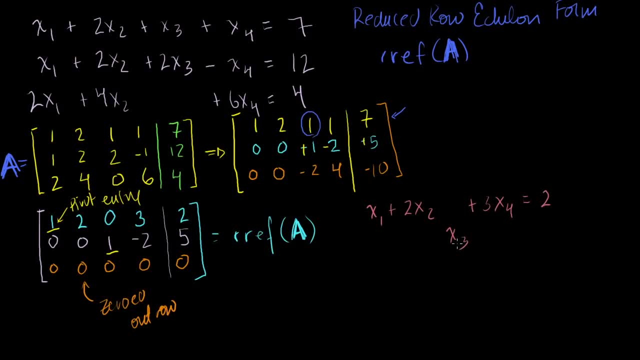 No x2.. I have an x3.. I have x3 minus 2x4 is equal to 5.. And then I have no other equation here. This one got completely zeroed out, So I was able to reduce this system of equations to this. 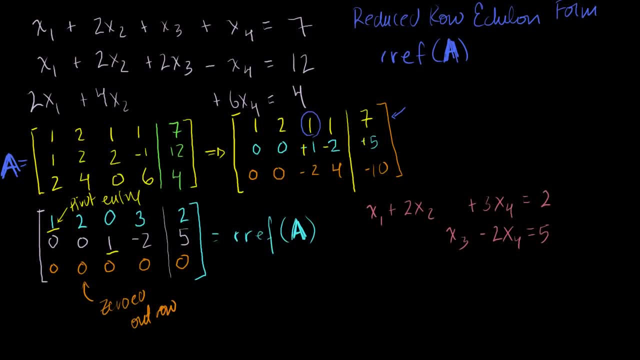 system of equations. Now the variables that you associate with your pivot entries, we call these pivot variables. So x1 and x3 are pivot variables- Pivot variables. And then the variables that aren't associated with a pivot entry, we call them free variables. 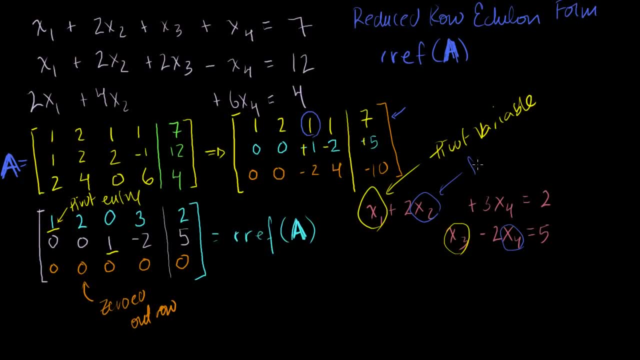 So x2 and x4 are free variables. But now let's solve for essentially you can only solve for your pivot variables, The free variables we can set to any variable, And I said that in the beginning of this equation. We have fewer equations than unknowns. so this is going to 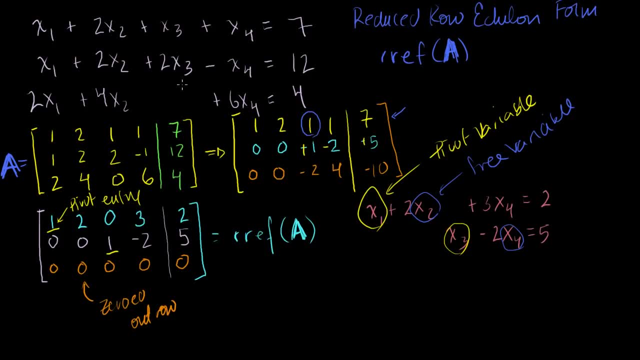 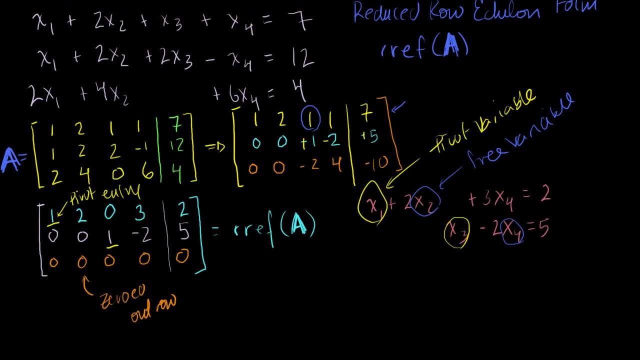 be not well constrained. OK Solution: You're not going to have just one point in R4 that solves this equation. You're going to have multiple points. So let's solve for our pivot variables, because that's all we can solve for. 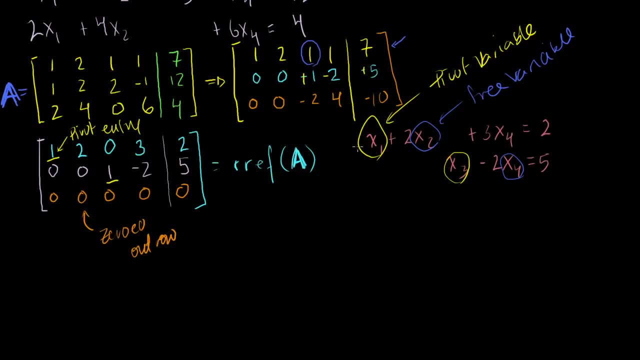 So this equation tells us, right here, It tells us x3.. Let me do it in a good color: x3 is equal to 5 plus 3.. And then we get: x1 is equal to 2 minus x2 plus minus 3x4.. 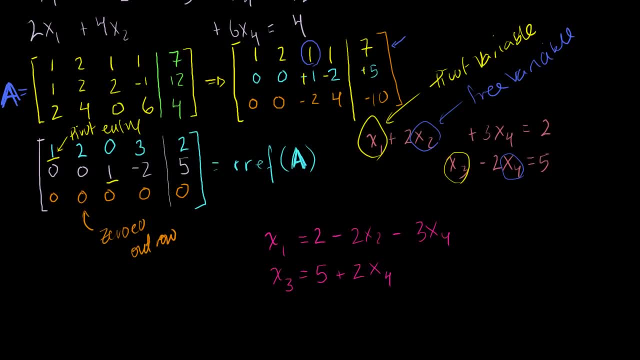 Right, I just subtracted these from both sides of the equation. Now, this right here is essentially as far as we can go to the solution of this system of equations. I can pick really any values for my free variables. I can pick any values for my x2's and my x4's and I can 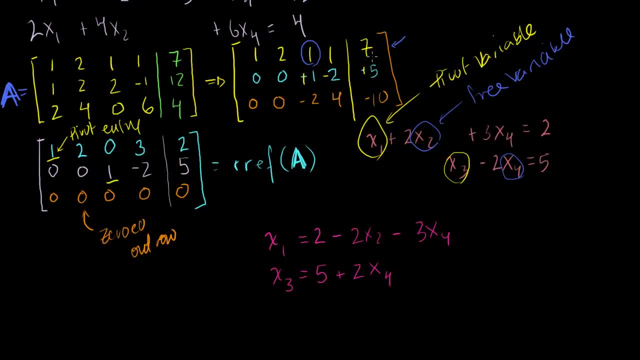 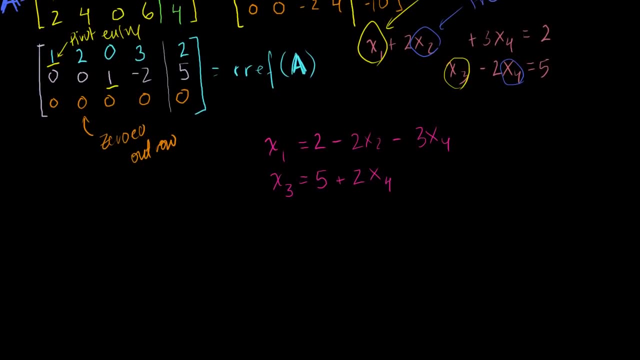 solve for an x3.. But what I want to do right now is write this in a slightly different form so that we can visualize a little bit better- And of course it's always hard to visualize things in four dimensions- but so we can visualize things a little bit. 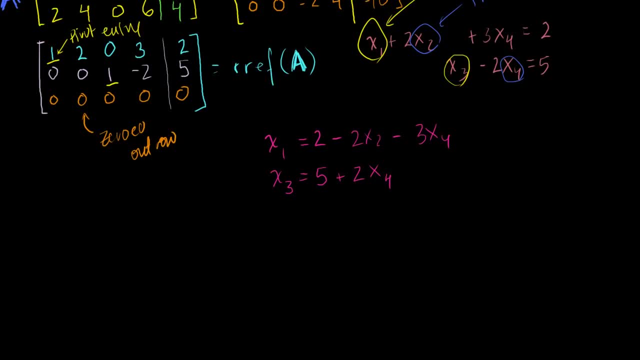 better as to kind of the set of this solution. So let's write it this way. If I were to write it in vector form, our solution is the vector x1, x2, x3, x4. And what is it equal to? 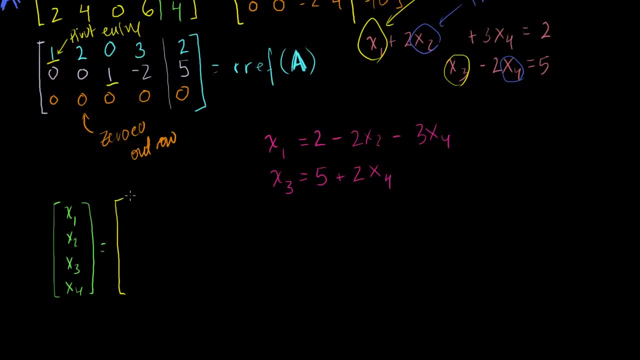 Let me write it like this: I'm just rewriting, I'm just essentially rewriting this solution set in vector form. So x1 is equal to 2.. Let me write a little column there: Plus x2.. Let me write it this way: 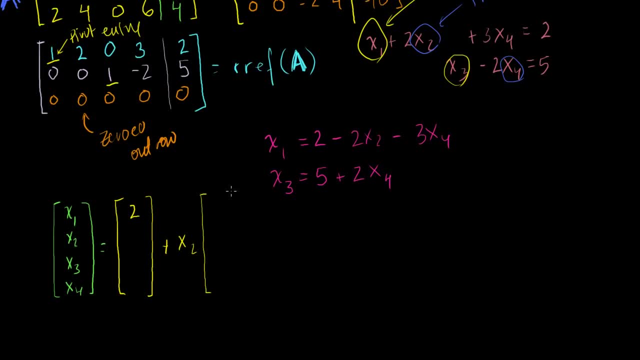 Plus x2 times something, Plus x4 times something. So x1 is equal to 2 minus 2 times x2. Or plus x2 times minus 2. So I put a minus 2 there And then I can say plus x4 times minus 3.. 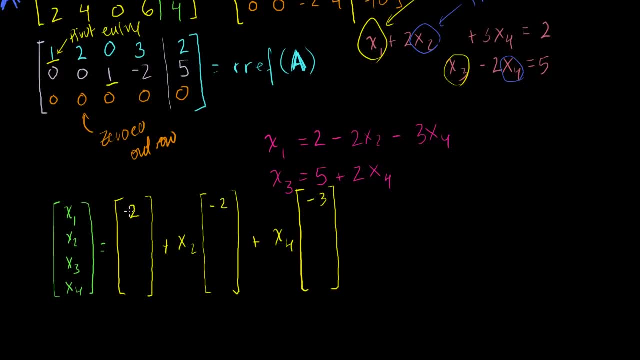 So I can put a minus 3 there. This, right here, these first entries of these vectors Just literally represent that equation. right there, x1 is equal to 2 plus x2 times minus 2 plus x4 times minus 3.. 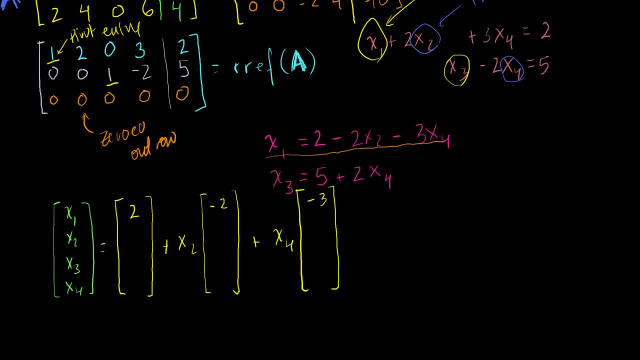 Now what does x3 equal? x3 is equal to 5.. Put that 5 right there. Plus x4 times 2.. Plus x4 times 2.. x2 doesn't apply to it, So we can just put a 0.. 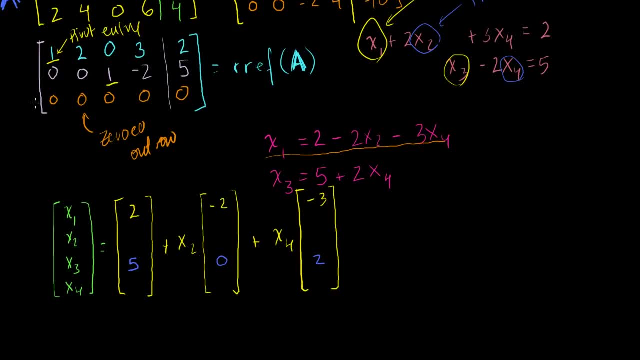 0 times x2.. Plus 2 times x4.. Now, what does x2 equal? Well, you could say: x2 is equal to 0 plus 1 times x2.. Plus 0 times x4.. x2 is just equal to x2.. 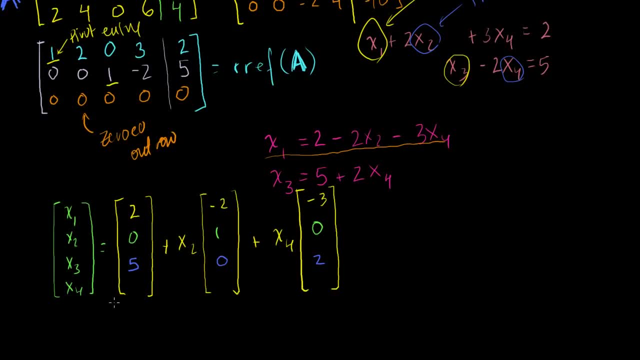 It's a free variable. And similarly, what is x4 equal to? x4 is equal to 0 plus 0 times x2 plus 1 times x4.. Now, what does this do for us? Well, all of a sudden, here we've expressed our solution. 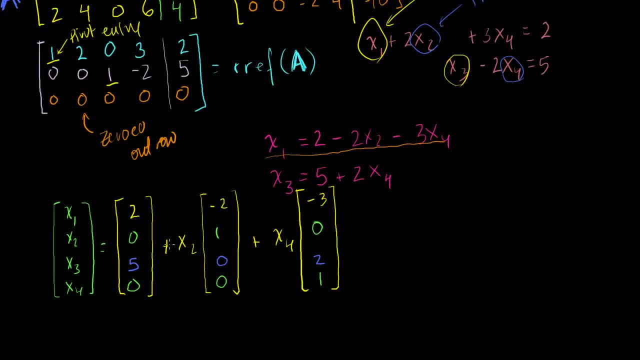 set as essentially the linear combination, Well, of the linear combination of three vectors. This is a vector in. you could view it as almost a coordinate in, either a position vector. It is a vector in R4.. You can view it as a position vector or a coordinate in R4.. 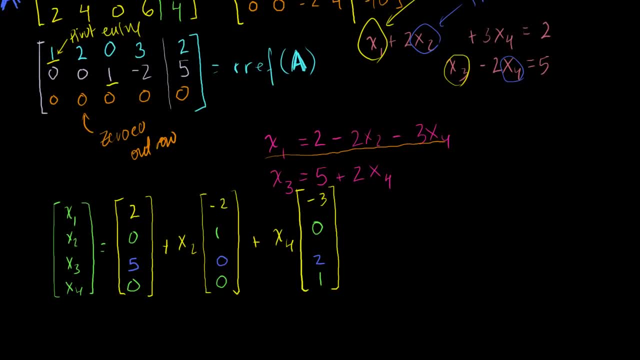 And then you could say: look, our solution set is essentially: this is in R4. Each of these have four components, But you could imagine it in R3. That I have, my solution set, is equal to some vector there that you know. that's the vector. 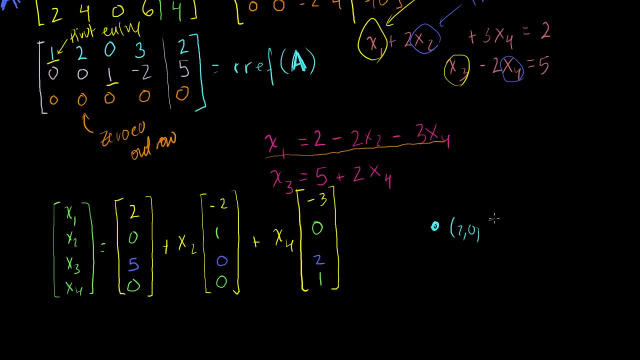 If you think of it as a position vector, it would be the coordinate 2 comma 0 comma 5 comma 0.. Which, obviously, this is four dimensions right there, But it's equal to multiples of these two vectors. So let's call this vector right here. let's call this vector. 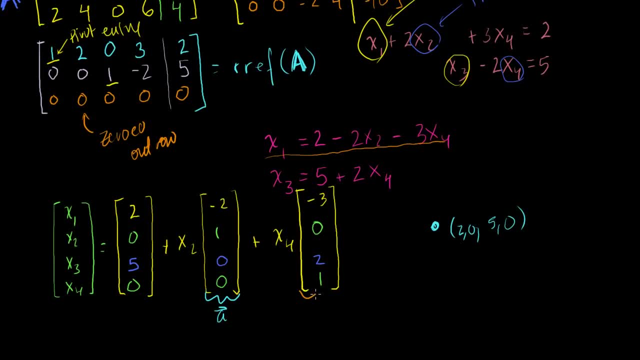 vector a, And let's call this vector, right here, vector b. So our solution set is all of this point, which is right there. Or I guess we could call it vector a, Or I guess we could call it vector b, Or I guess we could call it vector a. 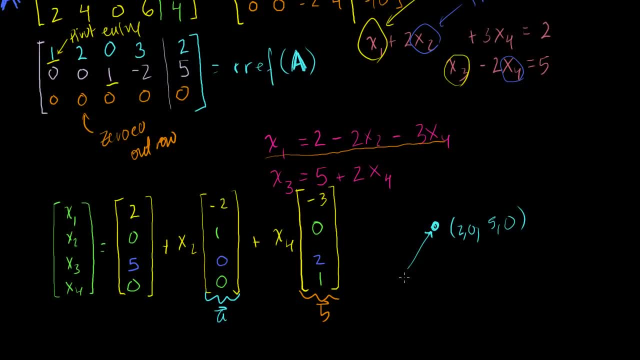 Or I guess we could call it that position vector, right? That position vector will look like that: Where you're starting at the origin, right there, Plus multiples of these two guys. So if this is vector a, let's do vector a in a different. 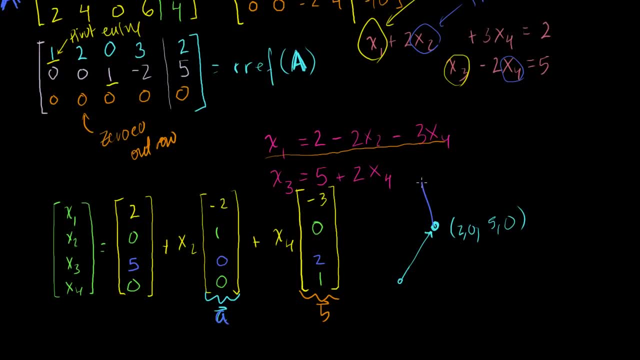 color. vector a looks like that. So let's say vector a looks like that, And then vector b looks like that. This is vector b and this is vector a, And I don't know if this is going to be easier or harder. 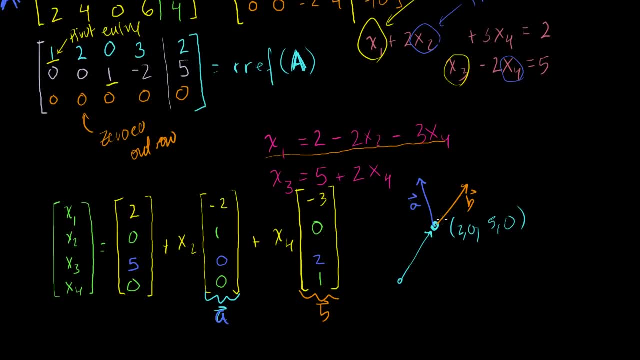 for you to visualize, because obviously we're dealing in four dimensions right here And I'm kind of just drawing it on a two-dimensional surface. But what you can imagine is that the solution set is equal to this fixed point, this position vector plus linear. 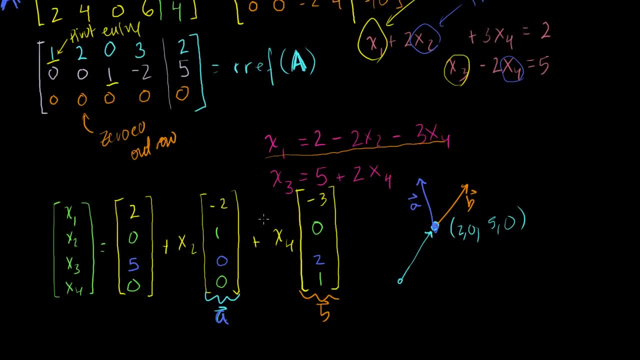 combinations of a and b And we're dealing, of course, in r4.. Let me write that down: We're dealing in r4.. But linear combinations of a and b are going to create a plane, right? You can just take. you know, you can multiply a times 2 and 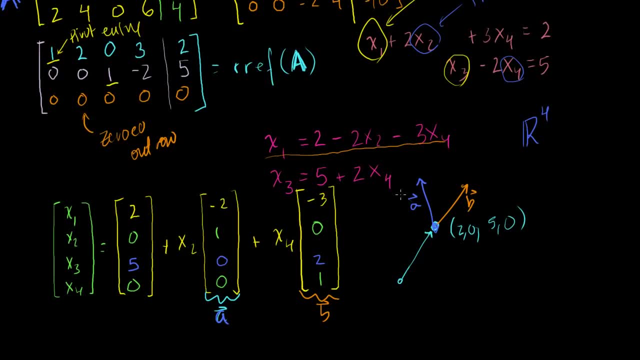 b times 3, or a times minus 1.. And b times minus 1.. And b times minus 100. And you can just keep adding and subtracting these linear combinations of a and b And they're going to construct a plane that contains the. 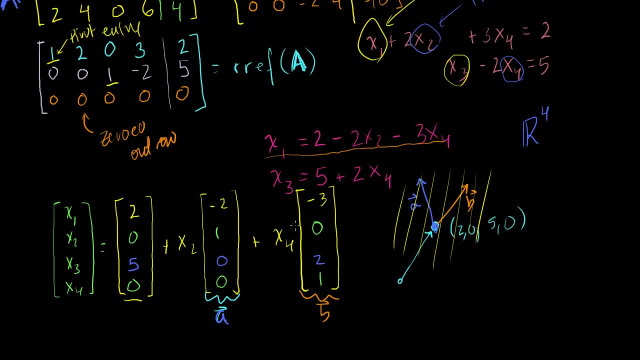 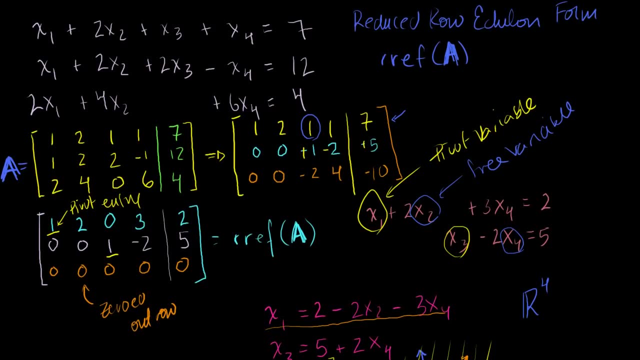 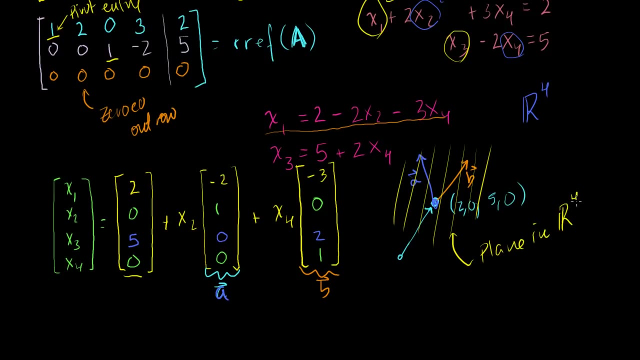 position vector, or that contains the point 2, 0,, 5, 0. So the solution for these three equations with four unknowns is a plane in r4. And I know that's really hard to visualize And maybe I'll do another one in three dimensions.